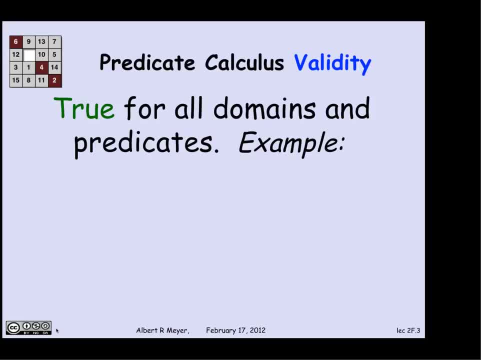 So a formula is valid if it comes out true, no matter what the predicate means. Let's look at it. I'll give you a concrete example to get a grip on this. Here is a valid formula of predicate calculus. It's mentioning predicates p and q. 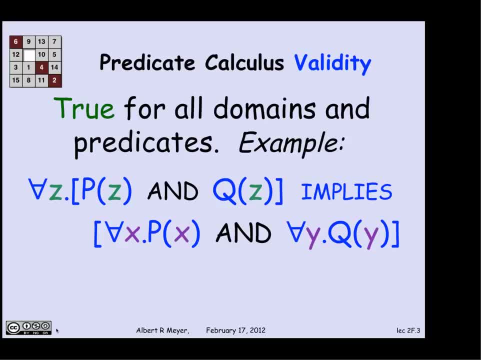 It's of the form of a proposition, because it's saying something about every possible z in the domain and every possible x and every possible y, The only thing that we need to know to make sense out of this formula, to figure out whether or not it's true. 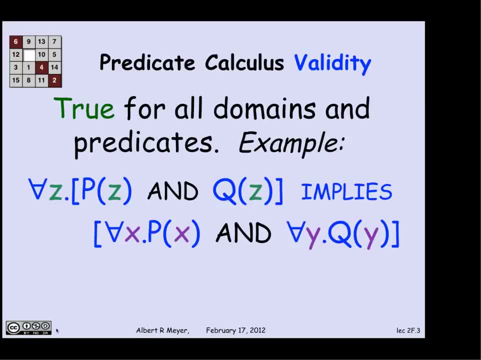 is: what's the domain that x, y and z range over, And what exactly do p and q mean? Well, I want to argue informally. Let's just look at what this is saying together. What this is saying is suppose that for everything. 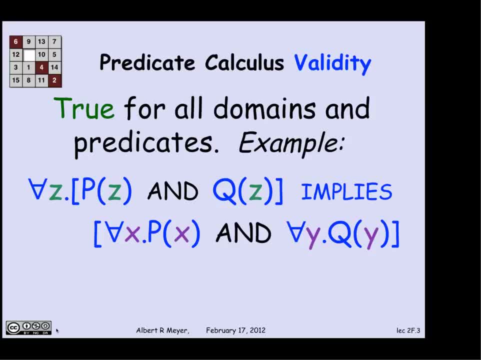 in the domain both property p of z and p of q, In other words, everything in the domain have property p and property q. Well, that certainly implies that everything in the domain has property p, because they have both properties, And also everything in the domain. 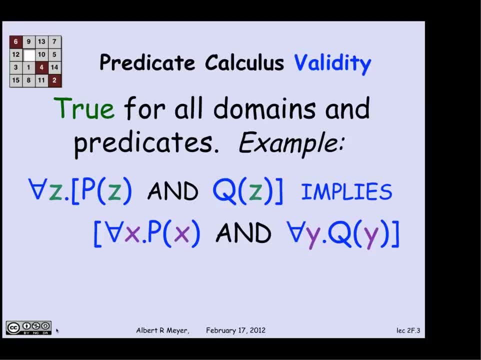 has property q, because everything has both properties. So when you say it that way, the sense that this is a fundamental logical fact that doesn't depend on what p and q mean or what the domain is, it's just a fact about the nature. 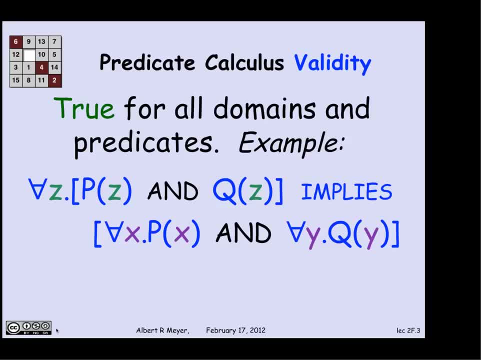 of the meaning of the for all universal quantifier and the connectives, and it implies. that's how we figure out that this is valid. Well, Let me go one level in more detail to say again what I just said informally and try to be a little bit more precise and clearer. 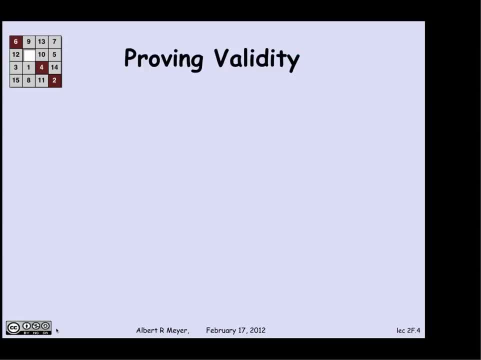 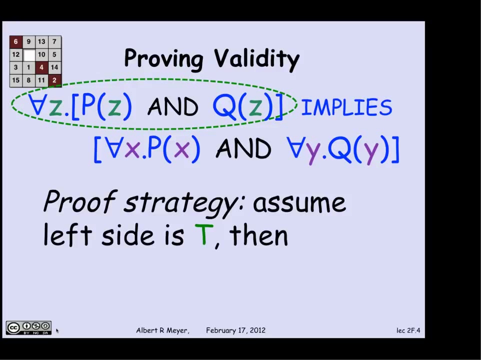 about a reason why this formula is valid. So suppose I wanted to prove that the formula is valid. Well, it's an implication. So the proof strategy. there it is written again, The proof strategy is, I'm going to assume that the if part, the left-hand side of the implies: 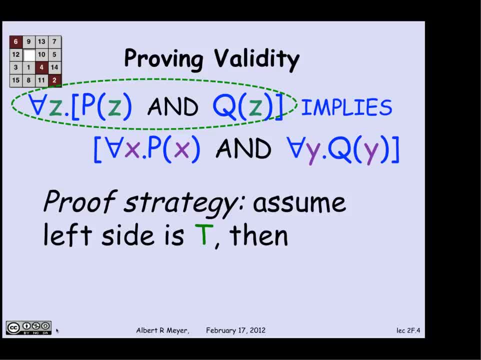 or hypothesis is true, That is, that for every z, p of z holds and q of z holds, And then I'm going to try to prove, based on that, that the consequent holds, namely that the right-hand side for all xp of x, 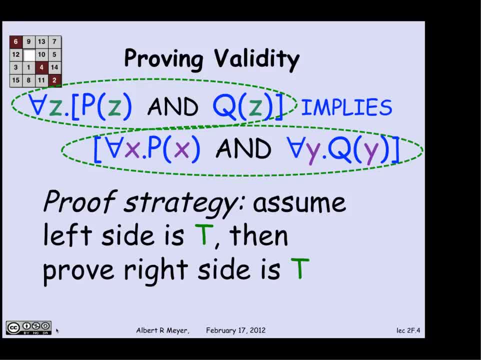 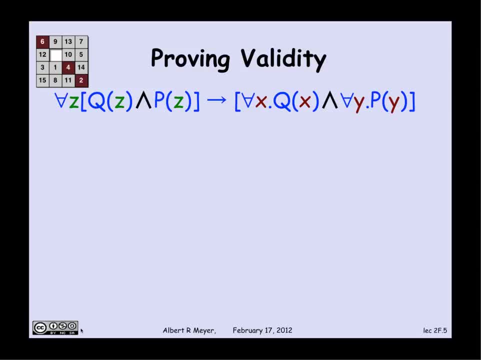 and for all y. q of y holds. OK, How am I going to do that? Well, so here's the formula, written just to fit on the line with the concise mathematical symbols: The upside down v means and, and the arrow means implies. 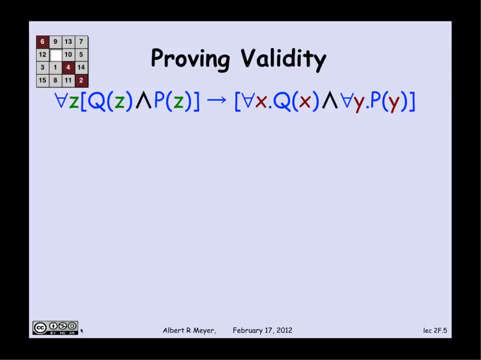 And we want to try to prove that this is validity, that this is valid a little bit more carefully. Well, the strategy, as I said, is to assume that the left-hand side holds. Well, what's the left-hand side say? 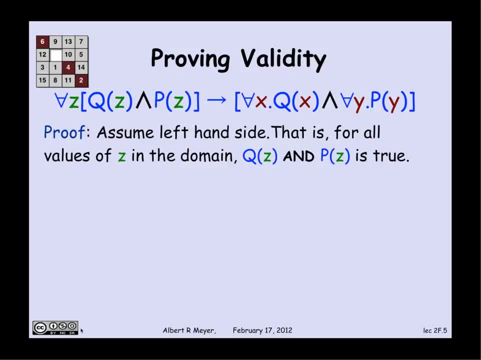 It says that for every z, q of z holds and p of z holds, That means that for every possible environment that assigns a value to z, q of z and p of z both come out to be true. Well, suppose that the value that the environment 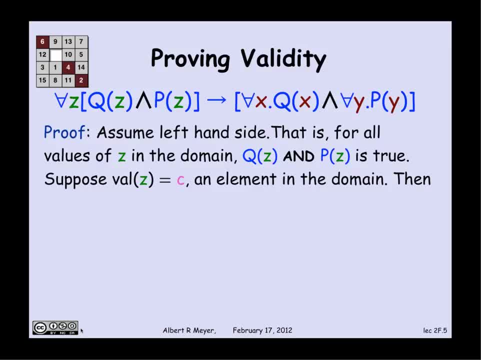 assigns the value c to z, where c is some element to the domain, Then what this means is that in that environment q of z and p of z is true, which means that q of c and p of c holds, But q of c holds, so q of c certainly holds. 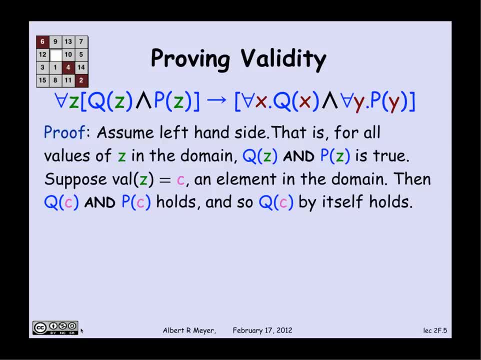 And p of c holds, so q of c certainly holds all by itself. All right, So now we're in an interesting situation because we just proved that q of c holds and we know nothing and have assumed nothing about c, except that it's an element to the domain. 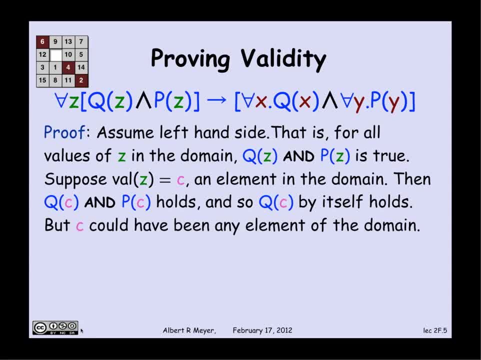 c could have been any element to the domain, And we've managed to prove that q of c holds, so it follows that in fact, we have really proved that for every x, q of x holds. Now that step of saying I proved it. 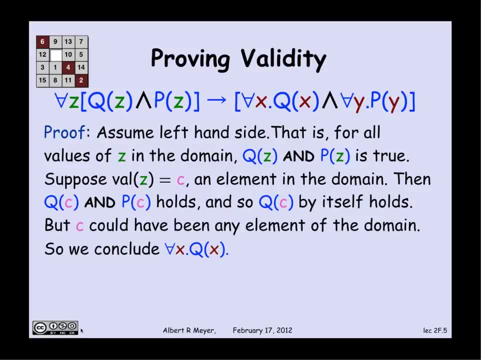 for q of a given element, without making any assumptions about the given element except that it's in the domain and therefore I can conclude that it holds, for all domain elements, very natural and plausible and understandable rule and it's a basic axiom of logic. 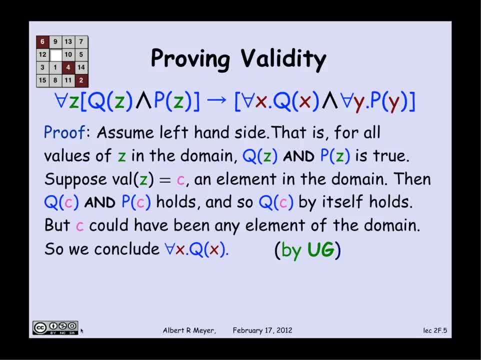 called UG, universal generalization. Come back to it in a minute. Anyway, I've just proved that for all x, q of x holds, and by a completely symmetric argument, for all y, p of y holds. and having proved both, for all x, q of x. 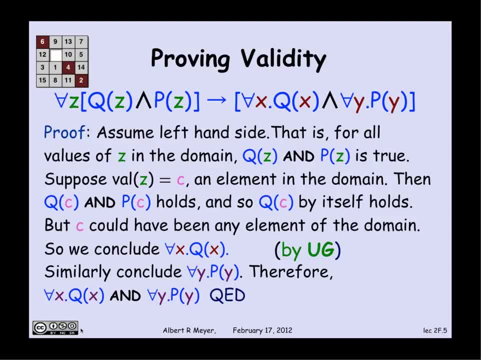 and for all y, p of y. clearly, the and holds- And I've just proved that the right-hand side of this implication is true, given that the left-hand side is true. Now, having called this proving validity, let me immediately clarify that this is not. 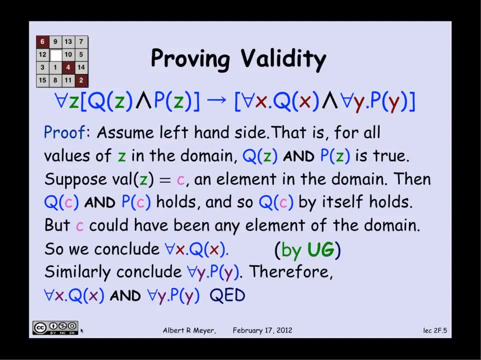 fair to call a proof, because the rules of the game are really murky here. This theorem you could read it as saying that universal quantification distributes over and is one of these basic, valid formulas that is so fundamental and intelligible that it's hard to see what more basic things 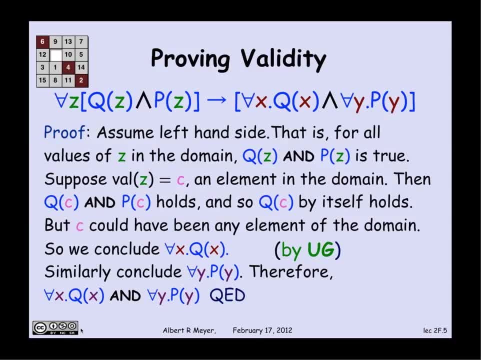 you are allowed to assume when you're proving it, and this proof really isn't anything more than translating upside-down A and the and symbol into English and saying that I'm using ordinary, intuitive rules about for all and and and using that in the proof. 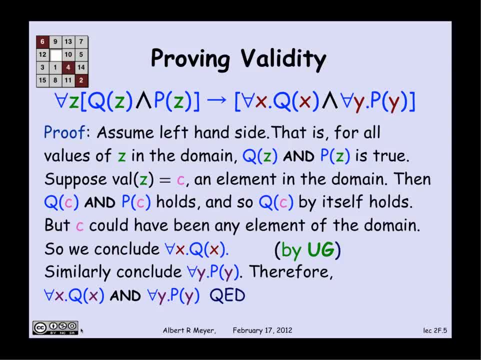 So this is a good way to think about the formula, to get an understanding of it, but it's not right to say that it's a proof OK, because we haven't been exactly clear about what the proof rules are And with this kind of really fundamental, valid fact, 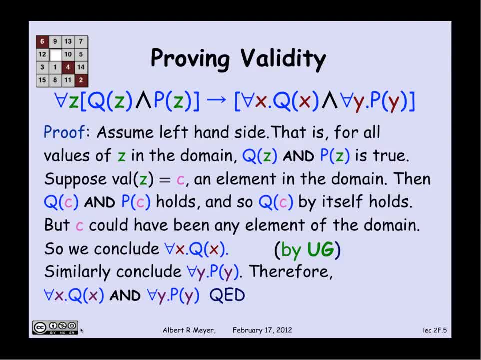 it becomes a quite technical problem to decide what a proof is going to be, what's fair to assume and what's fair not to assume. It would actually be perfectly plausible to take this as an axiom and then prove other things as a consequence of it. 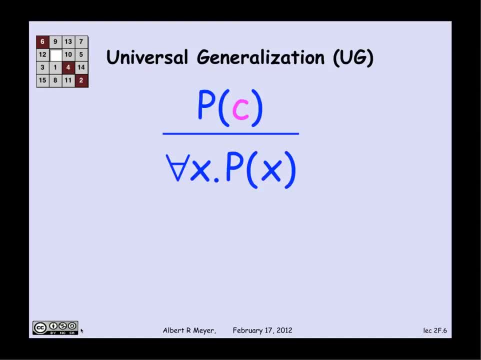 Anyway going on. let's look at this just for cultural reasons. We're never going to actually ask you to do anything with it, But the universal generalization rule, UG, would be stated this way as a deduction rule in logic. 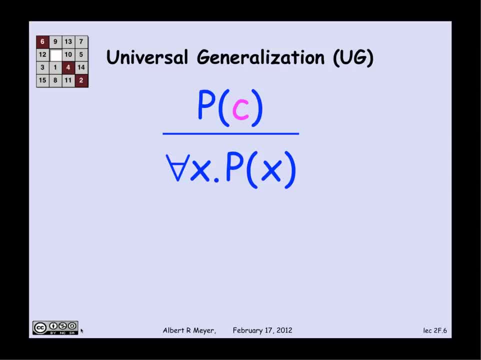 The stuff over the bar means: if you've proved this, then you can conclude that you've proved the stuff below the bar. So what this is saying is: if you've proved P of C for a constant C, then you can deduce that for every x, P of x holds. 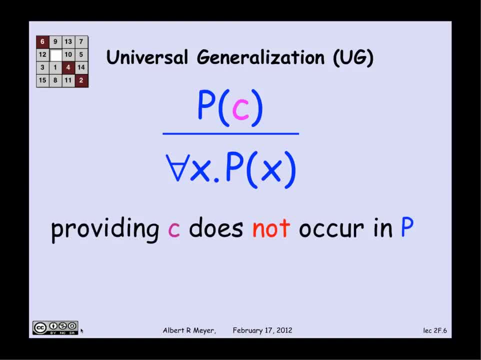 And this is providing that C does not occur in any other part of the predicate P, except where you're talking explicitly about it. It's hard to be more precise about that for now, Don't worry about it, But the idea is you're not supposed. 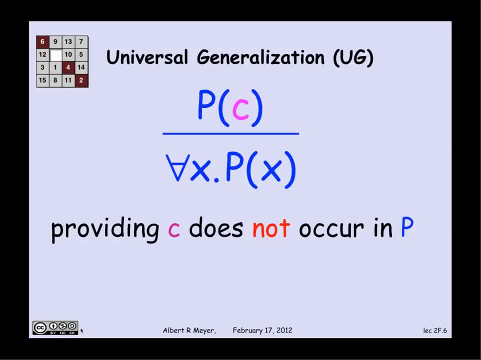 to assume anything about C other than it's in the domain and that it has property P, And you can then conclude that everything has property P. So let's look at a similar example. where it is possible to prove something Namely, I can prove that something's not valid. 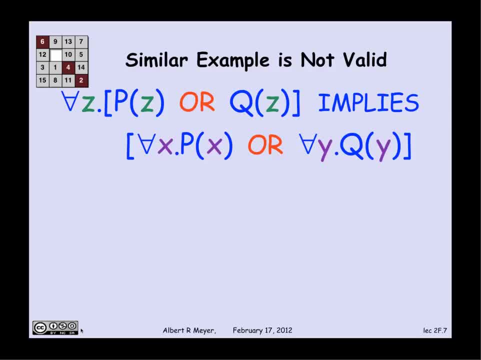 So here's a similar looking formula. This one says that for every z, if P of z holds or Q of z holds, then for every x P of x holds, or for every y, Q of y holds. And this one we're going to show is not valid. 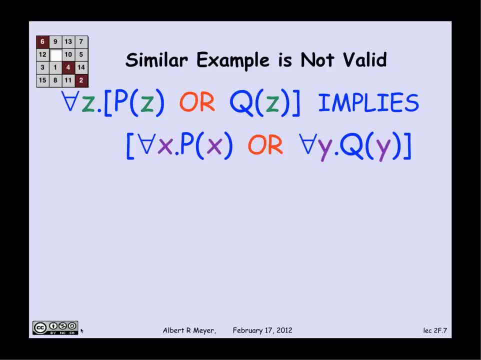 Let's think about it for a minute. What it's saying is: If everything has either property P or property Q, that implies that everything has property P or everything has property Q. Well, when you say it that way, it's clearly not the case. 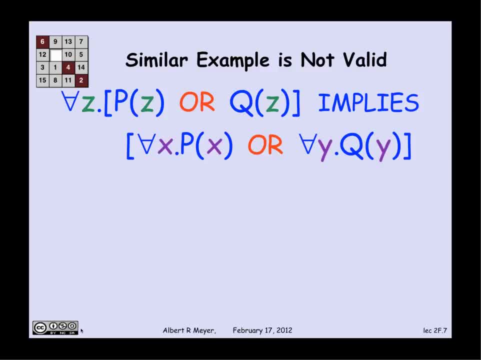 But let's go one level more precise and lay that out. What I'm going to do is convince you that it's not valid by giving you a counter model where I choose an interpretation, I choose a domain of discourse and predicates that Q and z are not valid. 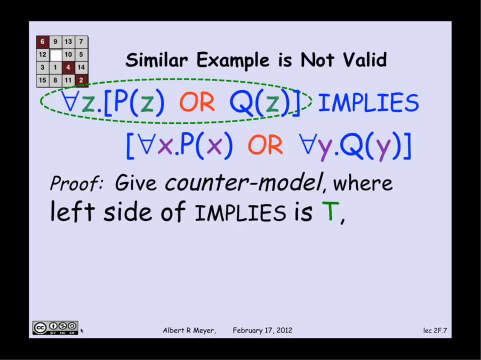 And that P and Q are going to mean over that domain And that make the left-hand side of this implication true. And then I'm going to show you that the right-hand side is not true And that means that in that domain, with those interpretations of P and Q, this implication fails. 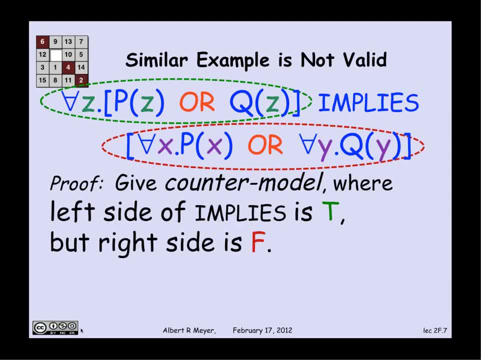 So it's not valid. So I need to make the left-hand side true and the right-hand side false. Well, I'm going to choose the domain of discourse to be the simplest one that will make this false, namely, let's let the domain of discourse just be the numbers 1 and 2..